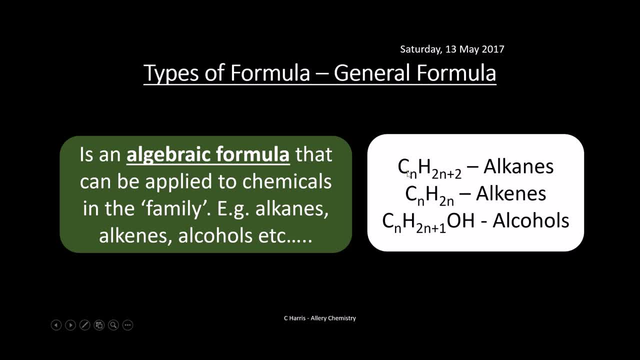 these are general formulas: CnH2n plus 2, where n is just the number of carbons. This is the general formula for alkanes. Alkenes with one double bond is CnH2n. Cytoalkanes also have this formula. 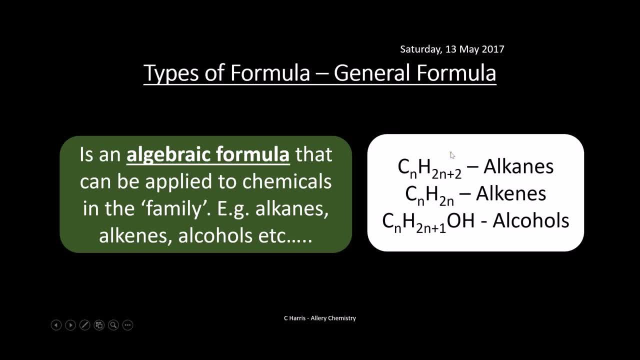 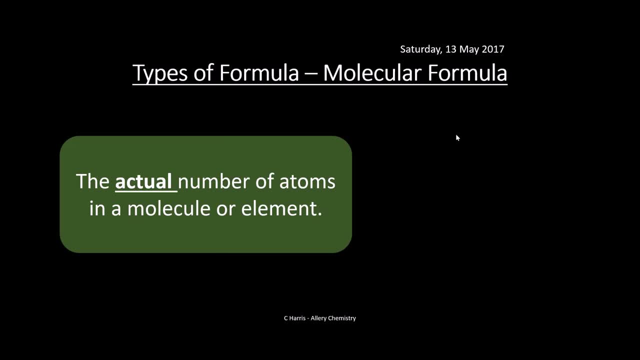 Alcohols, CnH2n plus 1.. So all these, basically, we can use these algebraic formulas to work out the formulas of any of these. Okay so molecular formula, So this is the actual number of atoms in a molecule or element. So, for example, ethane, C2.. 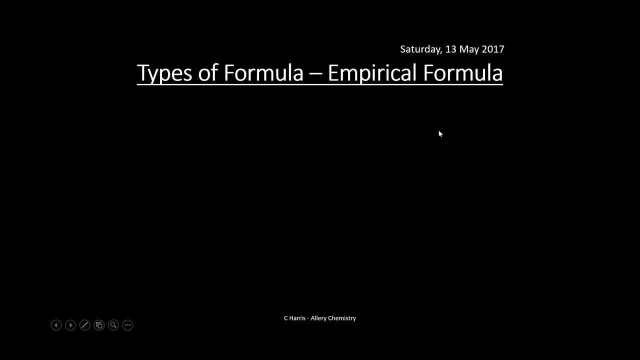 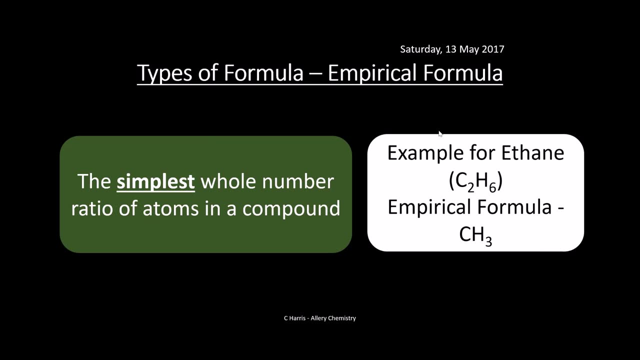 H6. So this is probably what you'll see quite often. Okay, empirical formula is the simplest whole number ratio of atoms in a compound. So empirical formula, for example, ethane, which is C2H6. That's the molecular formula, It's empirical formula. The simplest whole number ratio will be: 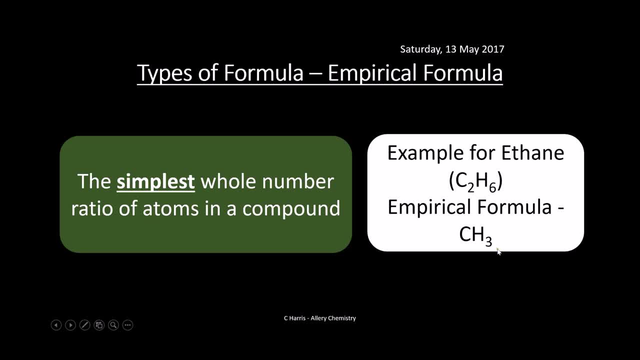 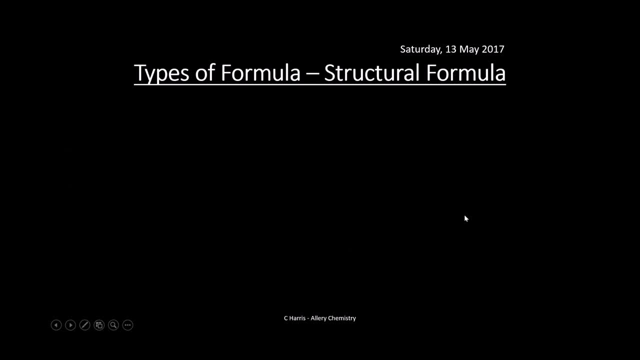 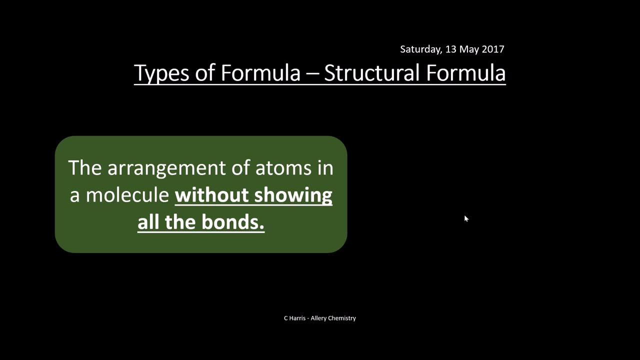 CH3.. Now, don't be worried about obviously this doesn't look right chemically right. Empirical formulas are just a whole number, ratio, So don't worry if it looks a bit bizarre, a bit strange. Okay, structural formula: This is the arrangement of atoms in a molecule, without showing all the bonds. Okay. so, for example, 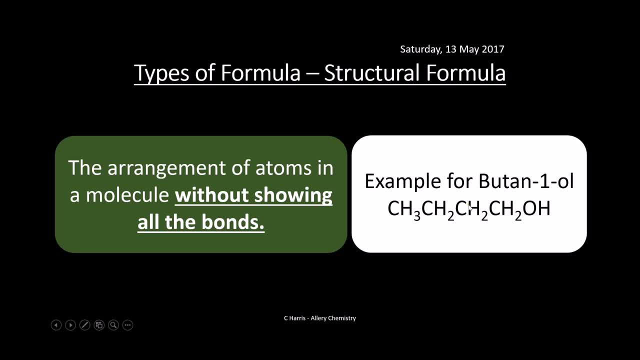 butane 1L. So we've got CH3.. CH2.. CH2.. CH2.. OH, So we've just chunked this molecule up. No bonds showing. That's an example for butane 1L, So a lot of the time you'll see it as CH3.. CH2.. CH2.. 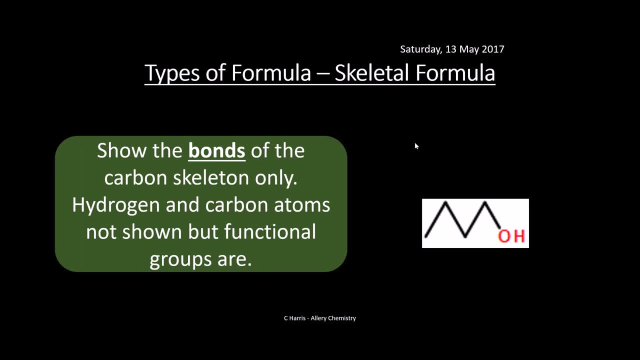 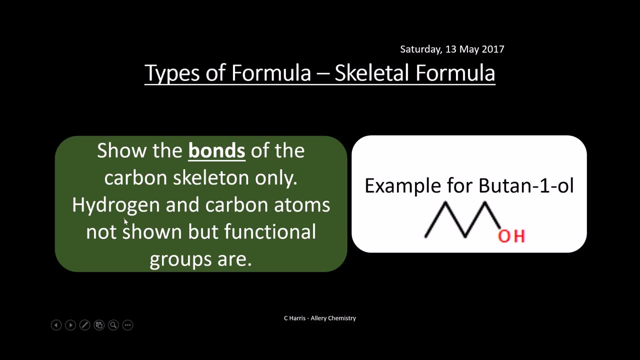 Things like that. Okay, so skeletal formula. Basically, these show the bonds of the carbon skeleton only, So hydrogen and carbon atoms are not shown, but the functional groups are, And they look a little bit like this. They look like zigzags And you see these quite often. It's just. 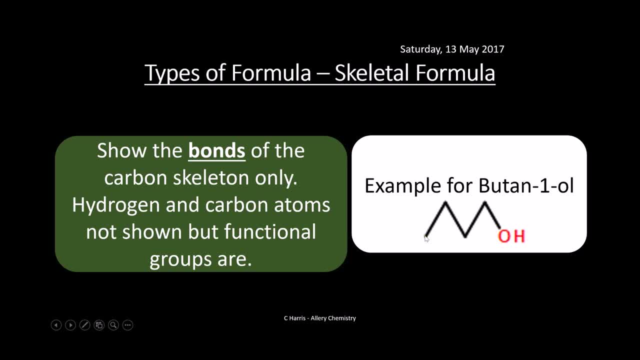 quicker to draw them. So this is butane 1L. You can see here we've got one, two, three, four carbons here. This carbon and the end, each point, represents a carbon. This carbon's got three hydrons attached. 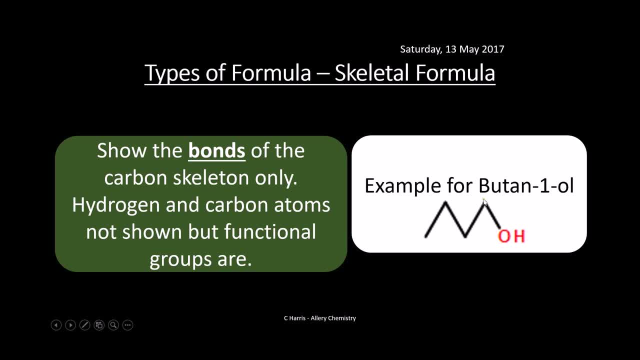 to it: This carbon's got two, This carbon's got two, That's got two as well. And then attached to it is an OH at the other side. So this is an example of a carbon skeleton. So, yeah, Okay, make sure you can draw these correctly And obviously each point is a carbon. 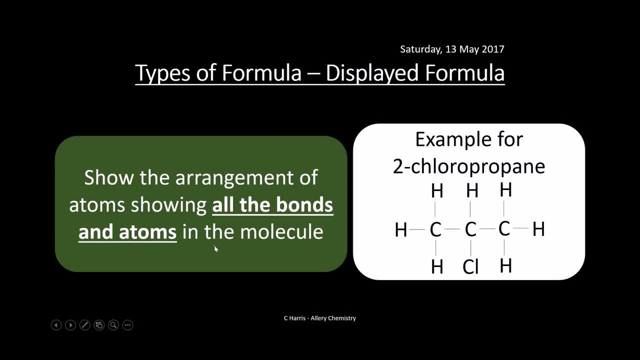 And displayed formula. Basically, these show the arrangement of atoms, showing all the bonds in an atom, in a molecule. So basically all your carbons, all your bonds, everything. So when it's asking for a displayed formula, make sure you draw it like this: So this is 2-chloropropane, Okay, so homologous series And you might. 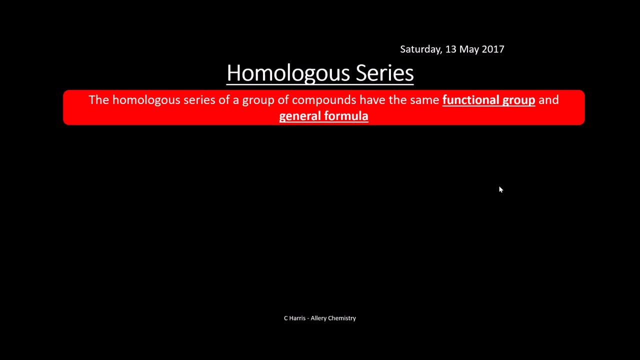 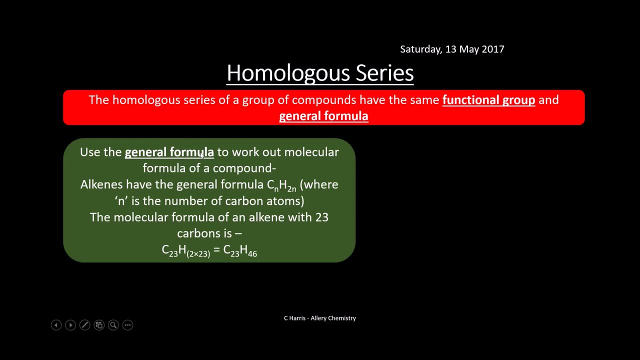 have seen this before. The homologous series of a group of compounds have the same functional group and general formula. So what we're going to do is use the general formula to work out the molecular formula of a compound. So alkenes have the general formula CnH2n. Okay, where n is the number of carbon. 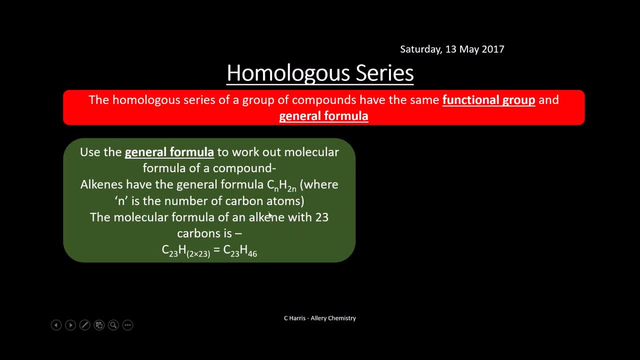 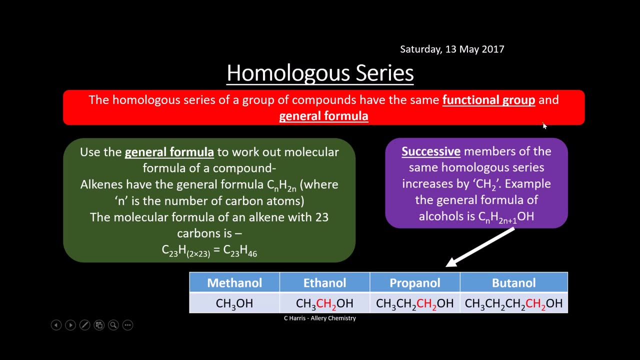 atoms And the molecular formula of an alkene with 23 carbons is C23H2L23. And this is going to be C23H46.. So this is just an example of an alkene general formula. So successive members of the same homologous. 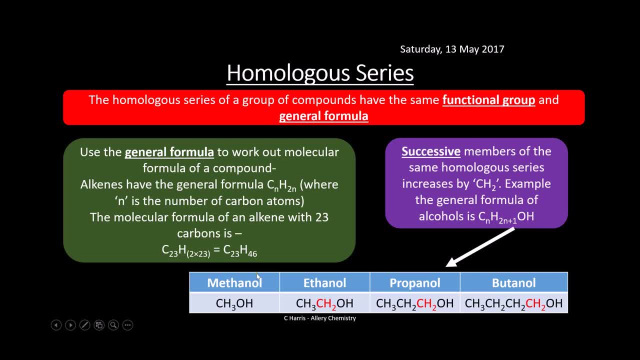 series increases by CH2.. So each time we're increasing it by CH2.. So the general formula of alcohols is CnH2n plus 1OH. Okay, and you can see here, So they've all got an OH, So they all belong. 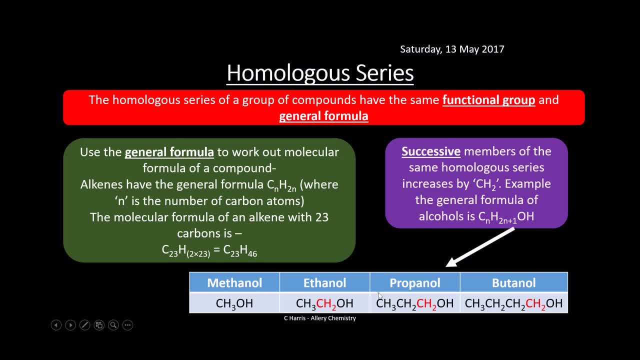 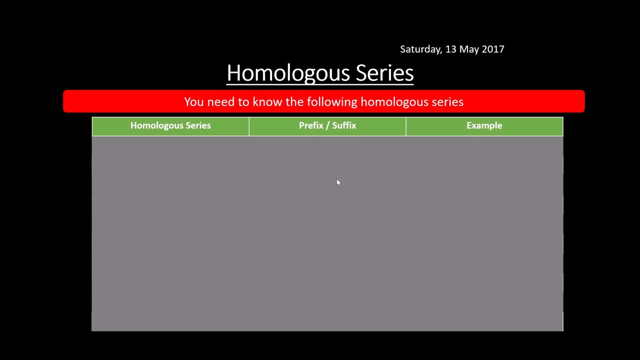 to the same homologous series. However, the difference is we're just increasing it by CH2.. As you can see in this example down at the bottom. Okay, so you need to know a few of these homologous series as well. So alkenes end in the word. 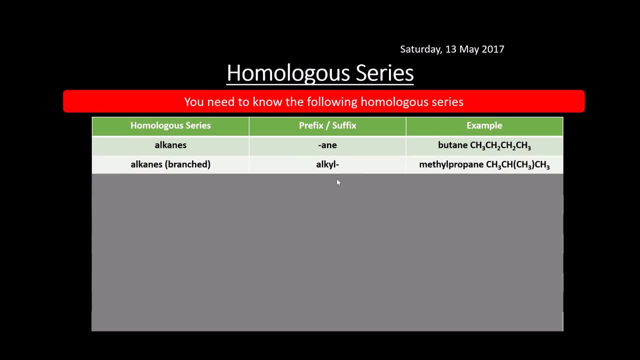 ane- And that would be an example- is butane. Alkenes that are branched have alkyl in them. So for example, methyl propane, It's got a methyl group hanging off of propane there. Alkenes end in ene. So that is propene. 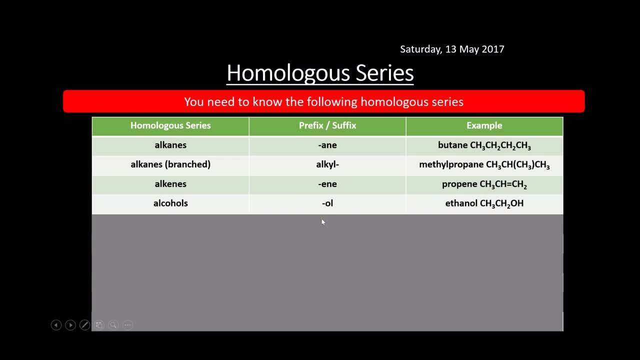 for example, Which is this one here: Alcohols end in ol, Ethanol. Okay, so it always ends in ol, And there's an example there. This is ethanol. here Aldehydes end in al, So, for example, propanal. You can see, here we've got this. 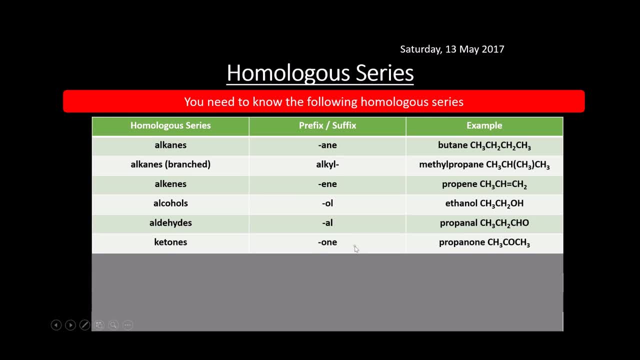 CHO at the end. there Ketones end in own. So there's propanone CH3, CO, CH3.. So you've got this very similar to an aldehyde. They have this C double bond O group Aldehydes are at the end Ketones. 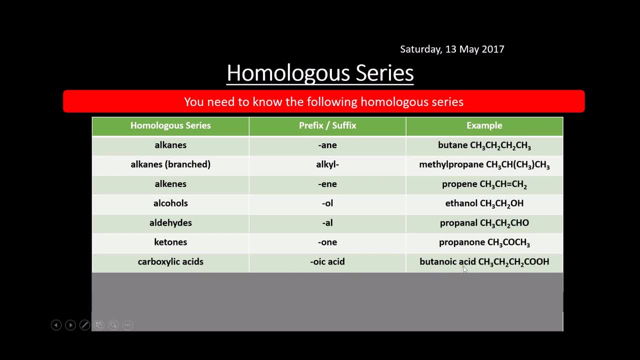 are in the middle. Carboxylic acids end in oic acid, For example, butanoic acid. So this is CH3, CH2, CH2, COA. This is butanoic acid. They always end in this COOH bit as well. Halogenol alkenes: These have a 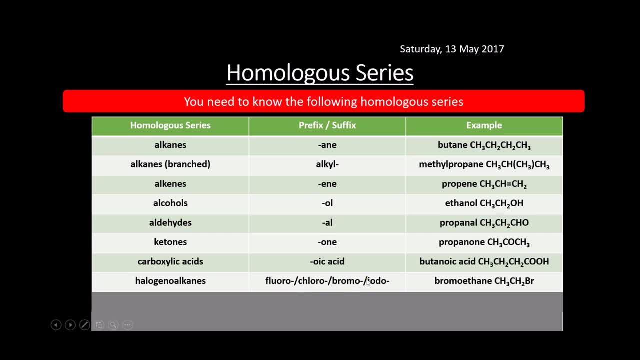 prefix. So these start as fluoro, chloro, bromo, iodo. So for example, bromoethane is CH3,, CH2, BR And chloro would just be chloromethane, chloroethane, etc. Cycloalkenes like we just 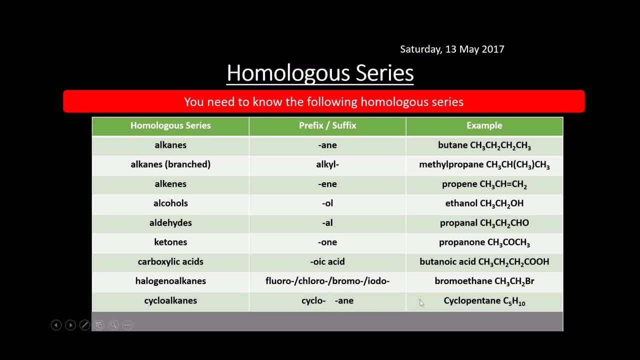 mentioned before. These start with cyclo and end in ene, So, for example, it's cyclopentane, So C5H10.. And esters: These start with alkyl, to start off with and end in anoate at the end. So 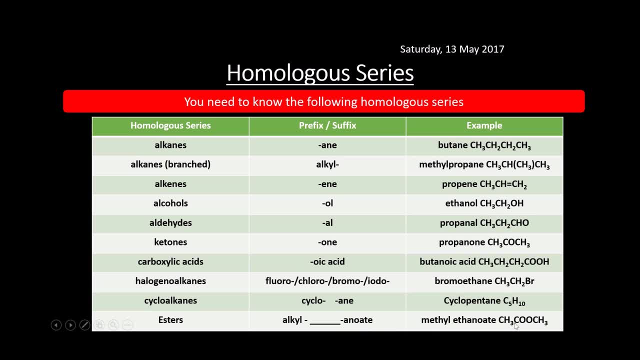 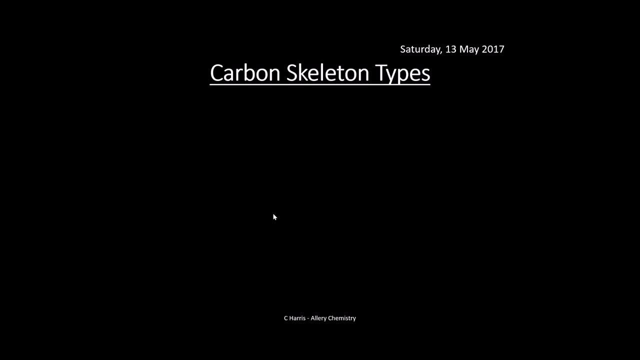 for example, methyl ethanoate- And this would be an example here- Very similar to a carboxylic acid, except instead of the H we have an alkyl group hanging at the end of it. Okay, so we need to know about a little bit more, about these carbon skeletons that we mentioned before. We need 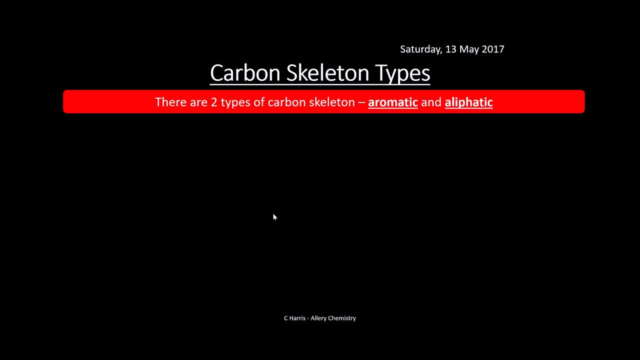 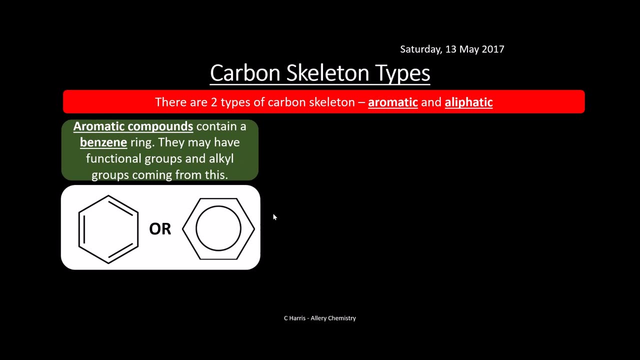 to know about the different types of them. Okay, So there's two types of carbon skeleton. We've got aromatic and aliphatic, Okay, And you've got very similar sounding words, but you've got to know the difference. So let's have a look at these. 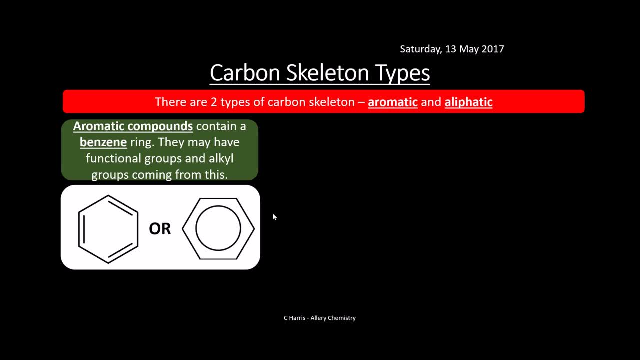 aromatics. first, These contain a benzene ring, Okay, And they may have functional groups and alkyl groups coming from them. So this is an example of an aromatic compound. They can either be just drawn like this or drawn like this. Aliphatic compounds, though, are straight chained. 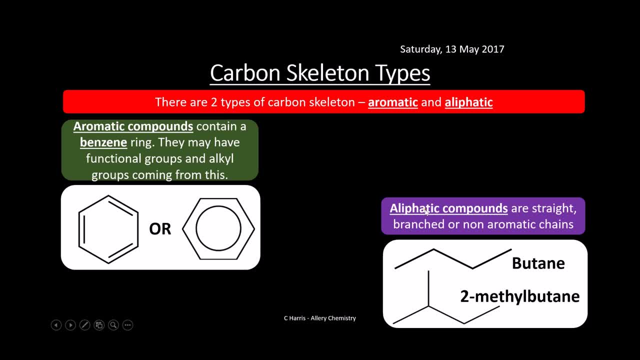 They're grouped in a ring like this. So you can see here, butane is an example of an aliphatic. 2-methylbutane is an example of an aliphatic chain, So these are not in a circle like benzene. 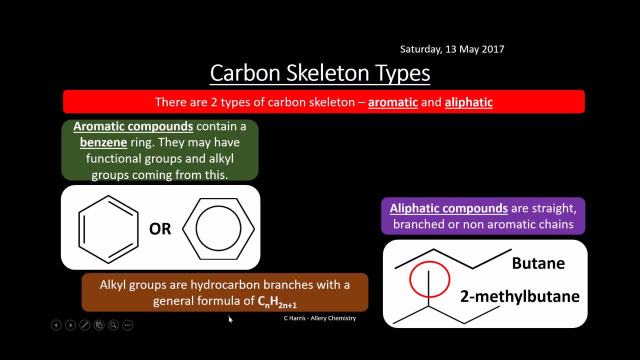 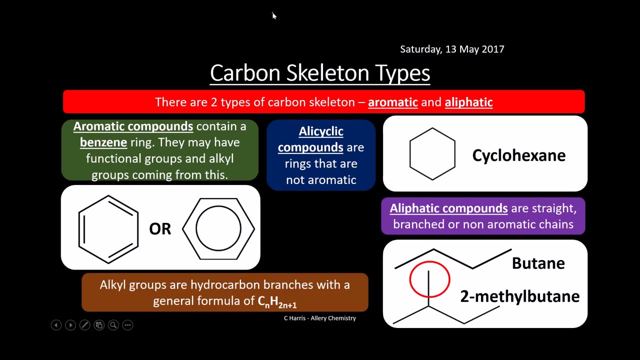 So alkyl groups are basically hydrocarbon branches and these always have this general formula here: CnH2n plus 1, because one of the spaces here has been used to bond with a carbon on the chain. Alicyclic compounds: These are basically rings that are not aromatic. So aromatics have three double bonds or circle. 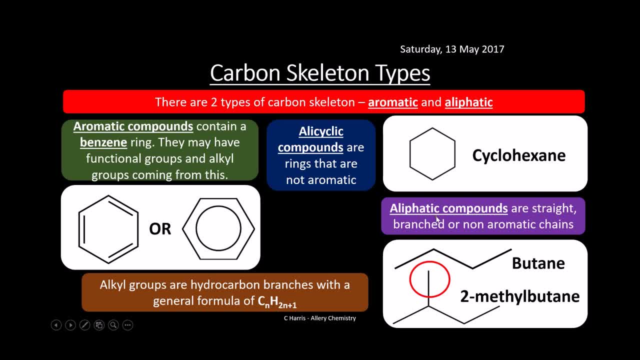 drawn in the middle. Alicyclics are basically aliphatic compounds, which is just straight chained hydrocarbon, except they loop together to form cyclo compounds, So it's like cyclohexane. So these are not aromatic. Don't get these two confused. They look similar, but aromatics, remember? 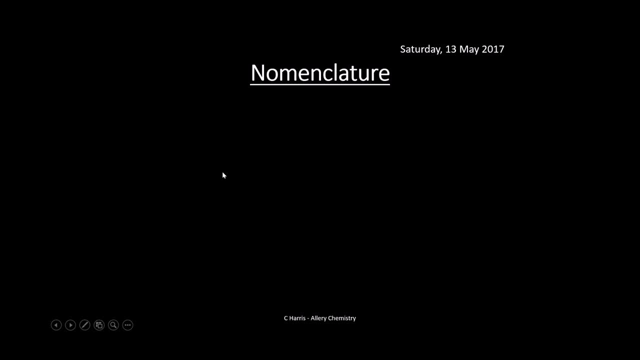 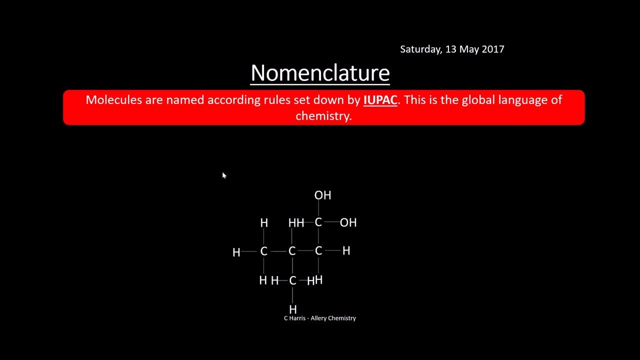 look for that circle in the middle. Okay, Nomenclature. This is probably one of the most important things you're ever going to do in organic chemistry is being able to name molecules, So you really do need to know these rules. Okay, so molecules are named according to. 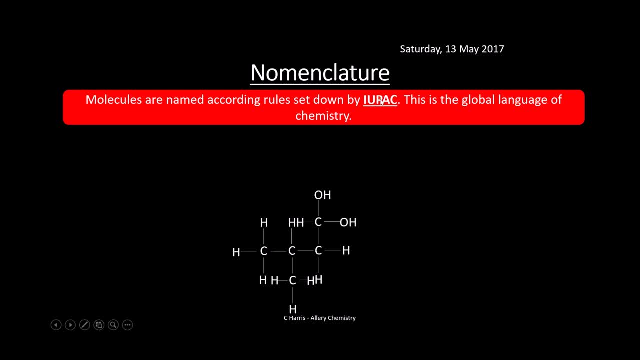 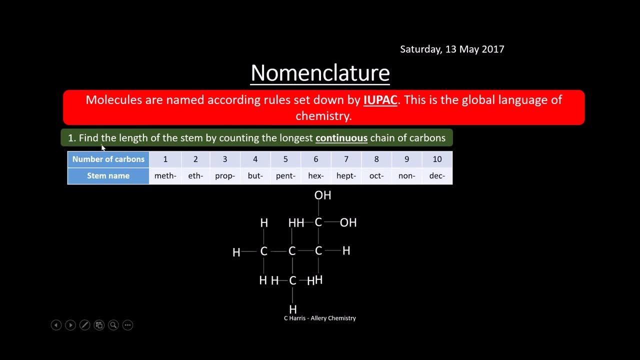 rules set down by IUPAC, which is the International Union of Pure and Applied Chemistry. Very catchy, isn't it? Okay, so this is the global language of chemistry. So the first thing we need to do is to find the length of the stem by counting the longest continuous chain of carbons. So you can see here. 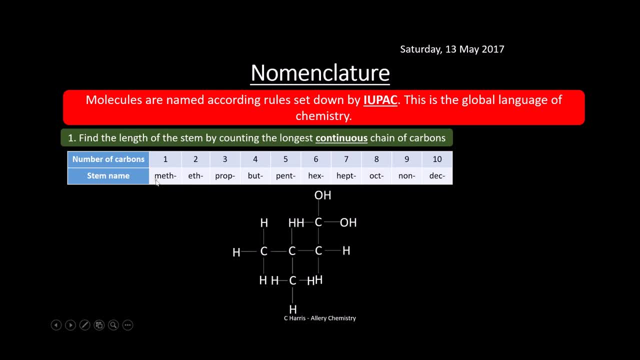 that we've got all these different prefixes here. It's the stem name. One is meth, two is eth, three is prop, four is, but five is pent, seven is pent and eight is pent, 6 is hex, 7 is hept, 8 is oct, 9 is non, 10 is dec. okay, so we're going to use some of these later. 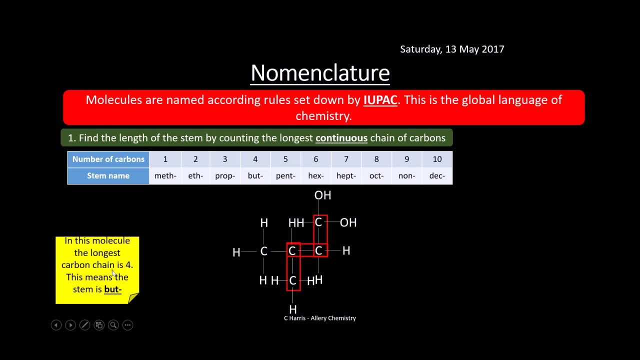 on. then, if we look at this molecule as an example, the longest carbon chain here is 4, so we're going to have butte as our stem name, okay, so the functional group on the molecule normally tells you the ending of the name, which is the suffix. so in this case this one has an oh on it. so this is going to end in all. okay, we've. 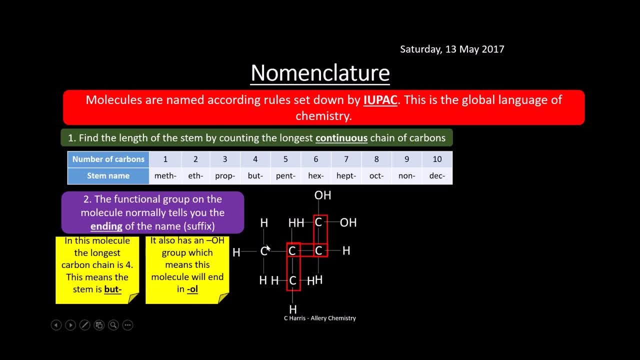 got two ohs on here, so this is going to end in all. so this is a type of alcohol. then the third thing we have to do is name a number, the carbon chain. so the functional group sits in the lowest possible number, carbon. so in this example, obviously the functional groups can sit on the first carbon. 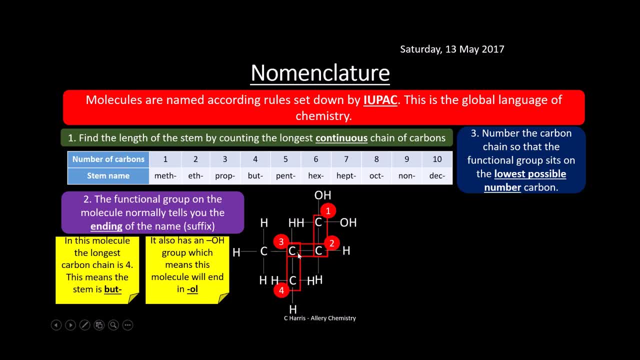 here, carbon number one. if i numbered it the other way, go one, two, three, four, then it means that the fourth carbon would have the two functional groups on and that is obviously bigger than one. so we always know number with the lowest number possible. then number four. what we do is we make a note of the carbon number. 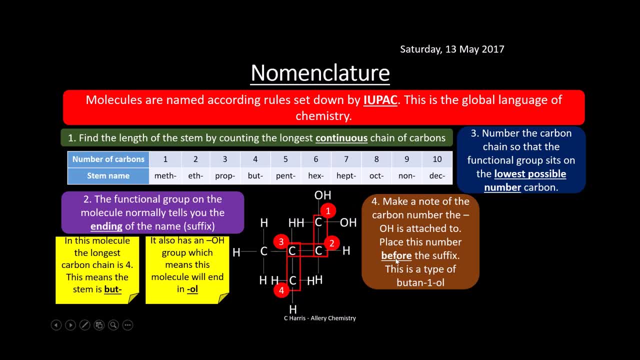 the oh is attached to. so this is carbon number one. place this number before the suffix um and this is a type of butan one, all this one, because we know it's butte, we know it's an alcohol and we know that the alcohol is on the first carbon. so any side chains and, less important, functional. 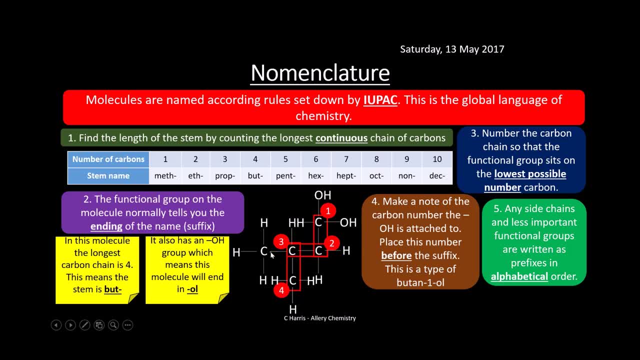 groups are written as prefixes in alphabetical order. see, here we've got a side group, here a methyl group hanging off here, off the third carbon, carbon number three. and if there is more than one, or if there are more than one identical functional groups either side, then we put di tri. 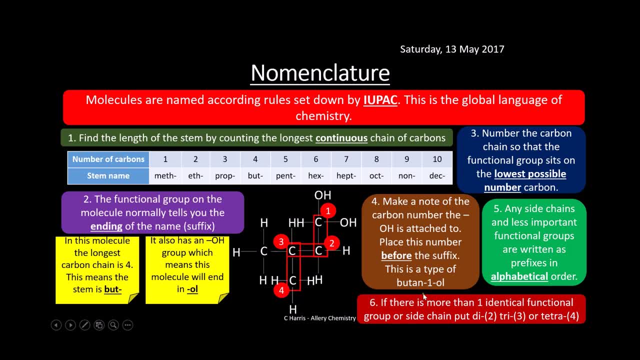 or tetra, and you can see here that we do have actually two alcohol groups. so we're going to put the word die in front of that to make it into two. so the name of this thing is called three methyl, because we've got a methyl group hanging off. the third, carbon butan, because you've got 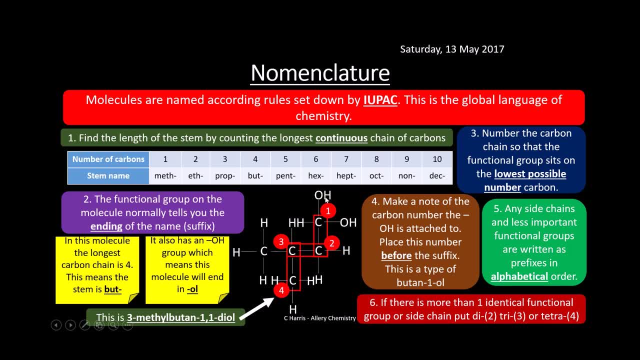 four carbons in the chain here, one, one, and then we've got a methyl group hanging off the third carbon, diol, because we've got two alls alcohol groups here, and it's die, because you've got two of them, so it's diol. and one one tells us that both of these are sitting on the first carbon, so it's. 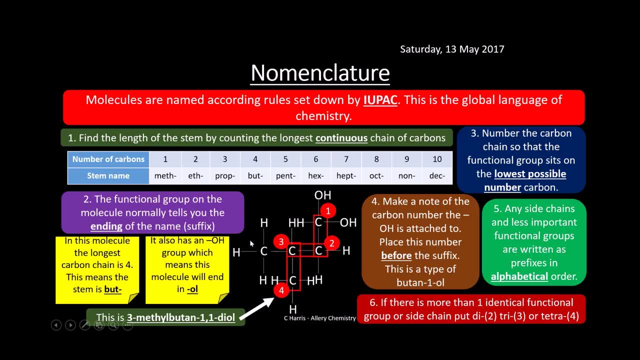 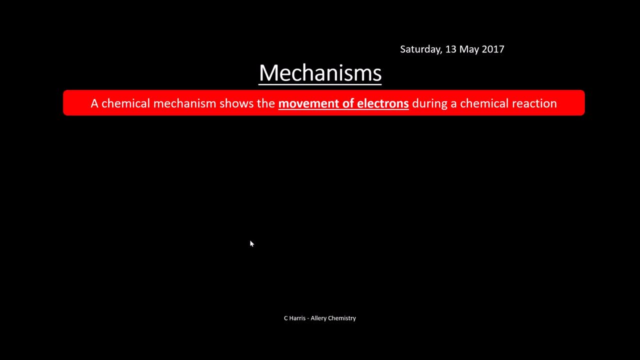 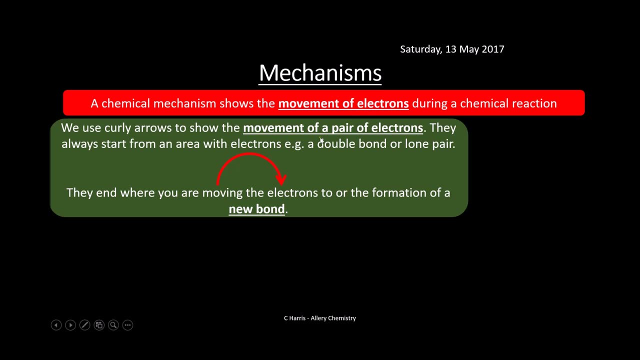 pretty much as simple as that. so make sure you know this dimension. it's so, so important. okay, mechanisms: obviously in organic chemistry you will see a lot of mechanisms going on here. so basically, this just shows you the movement of electrons during a chemical reaction. so we can use curly arrows to show the movement of a pair of electrons. 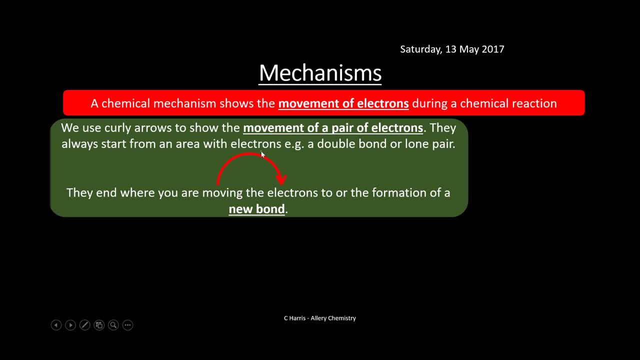 and so they all come together, and they all come together, and they all come together, and they all always start from an area where there is loads of electrons, for example the double bond or lone pair, and they end up moving the electrons to either form a new bond and or you can use them to break. 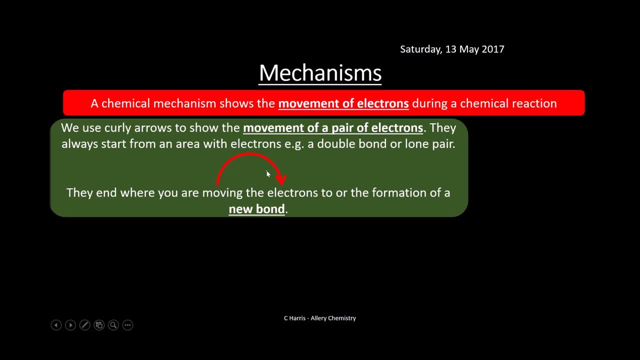 a bond as well, actually, and you can use them moving electrons from a bond onto an atom, for example. okay, you'll see some free radical mechanisms as well, but don't worry, don't need to know the curly arrows for them, so they're a bit different in terms of their mechanism. okay, so a 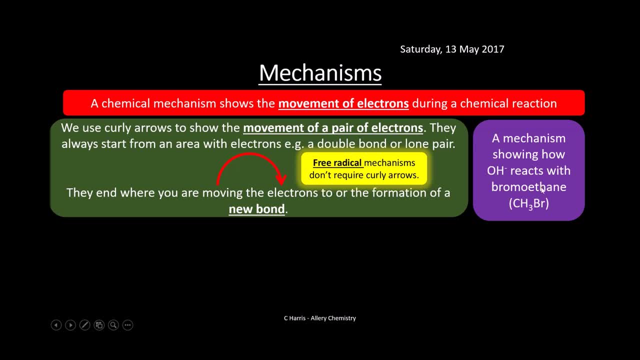 mechanism showing how oh minus reacts with bromo ethane. okay, so we're going to look at see what this is. so here is our bromo ethane. here one bromo ethane. there is an oh minus i, and i'm just going to show you, basically, how we can use these curly arrows to show how a reaction proceeds. so these 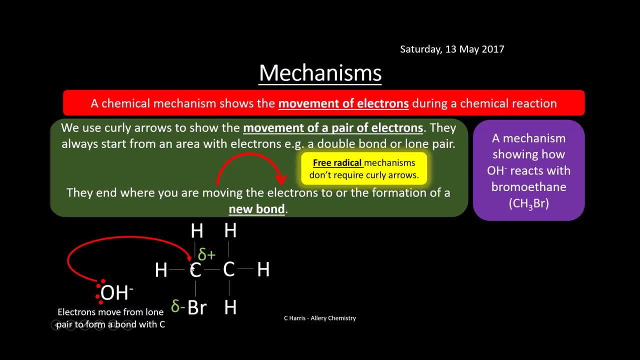 electrons are going to move from these lone pairs here and it's going to form a bond with carbon. this is what this arrow means: we're forming a bond with carbon. this one is basically showing the electrons breaking. this is what i'm saying here. so we're going to show you how the electrons are. 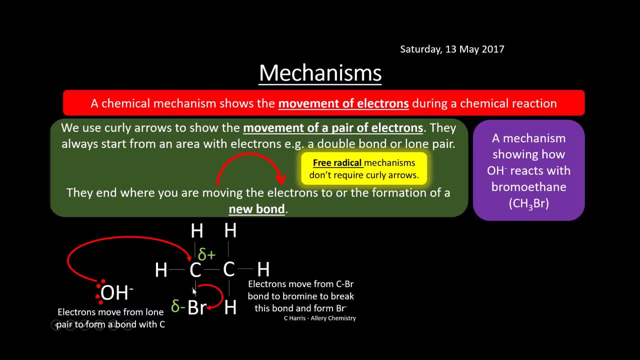 moving from a bond into the bromine. so this is the breaking of electrons. so remember, the arrow shows the direction of electrons. loads of electrons in the bond move into the bromine and this is going to form an alcohol in this case, and you can see here that the oh is now bonded to. 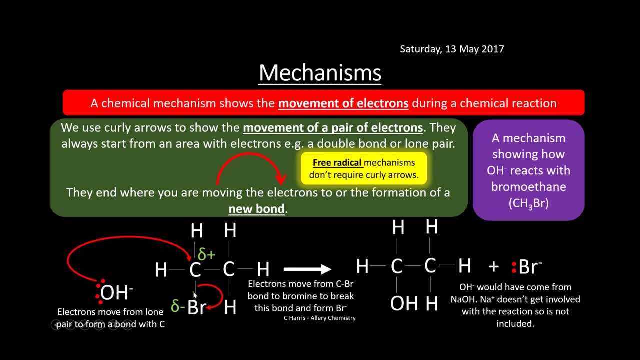 the carbon. there it is, but the bromine has been severed. the bond between the carbon, the bromine, has now broken and we have bromide ions that are left behind. um, so, yes, so not too much of a too bad. make sure you know what these arrows mean, because you're going to see a lot of them in. 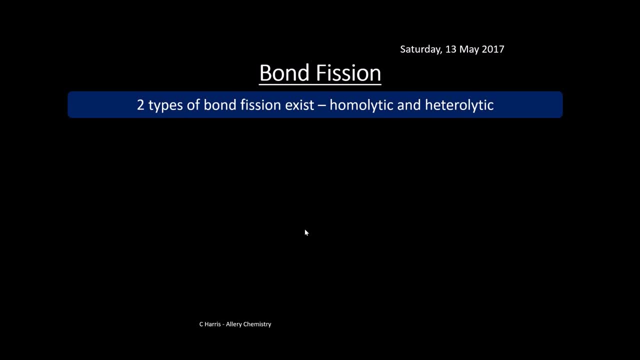 organic chemistry. uh right, bond fission. so there's two types of bond fission that exist. we've got homolytic and heterolytic, and we need to know the difference between them. okay, so bond fission is the breaking of a covalent bond. okay, so the electron pair and the bond can be distributed. 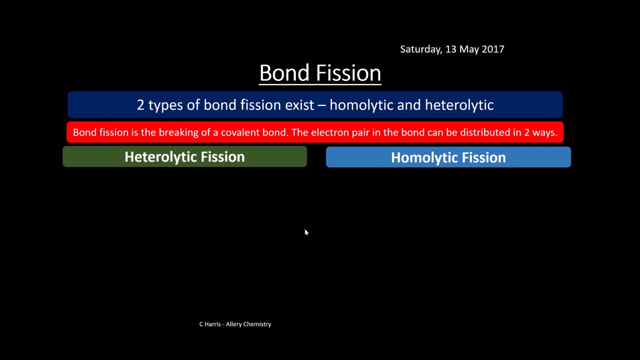 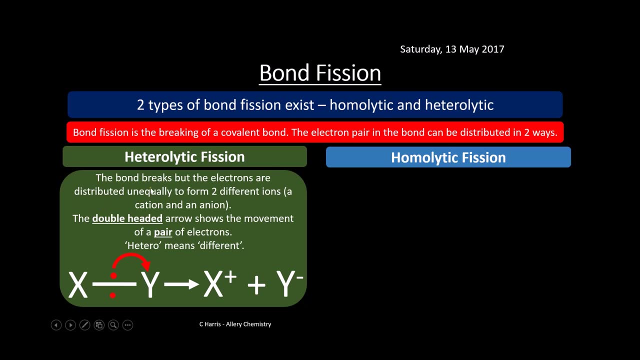 in two ways, so we can have heterolytic and homolytic fission. so let's start with. heterolytic is where the bond breaks but the electrons are distributed unequally. okay to form two different ions. so, um, we get a cation and an anion, so we've got a double-headed arrow shows the movement of. 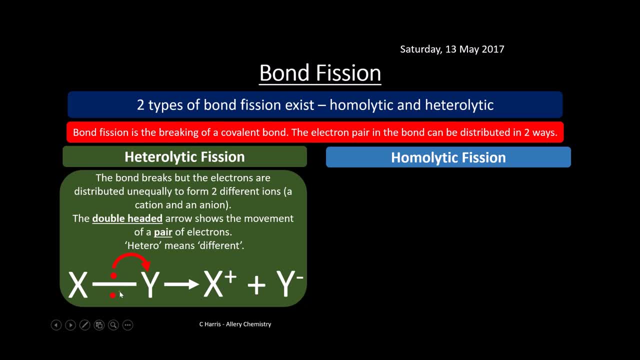 a pair of electrons. hetero means different, so you can see here that we've got these lone pair, well, sorry, bonding pair. here the electrons move onto one of the atoms, so what we're left with is that amp with a negative charge, and the one that's lost out on the electrons will have a 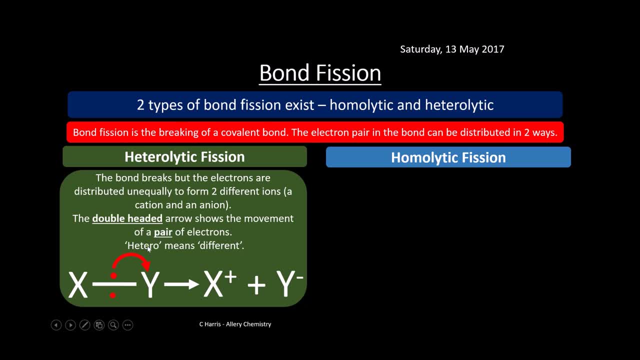 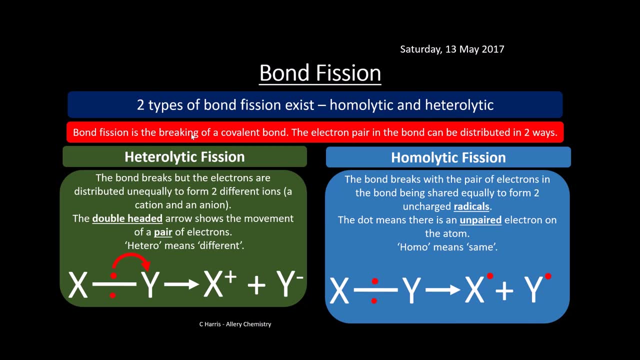 negative charge. they are different ions, so that's why we say they are heterolytic fission. homolytic fission is where the bond breaks, with the pair of electrons in the bond being shared equally to form two uncharged radicals. so the dot means there's an unpaired electron on the atom and 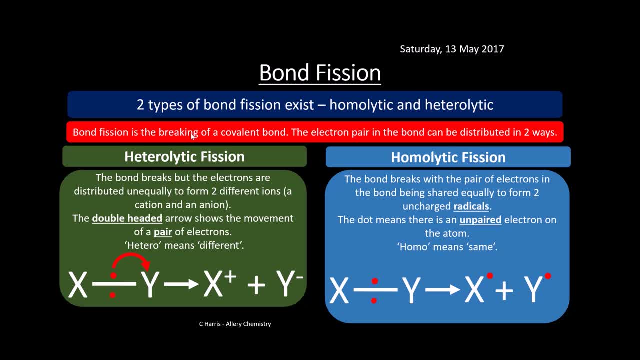 again. homo means the same, so we've got the same products are being produced. so here we've got x and y again with the lone pair, so with the bond pair in there, and basically what's going to happen is one electron is going to go on the y, the other electron is going to go on the x, and so we've got. 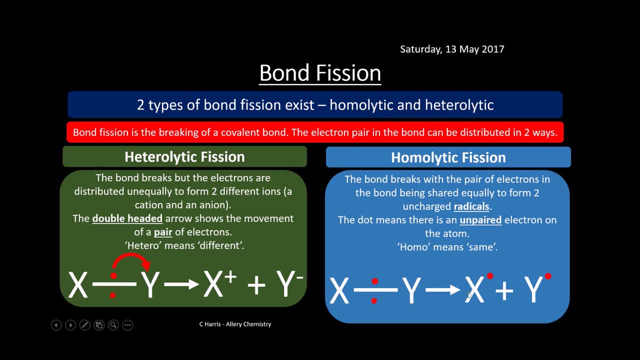 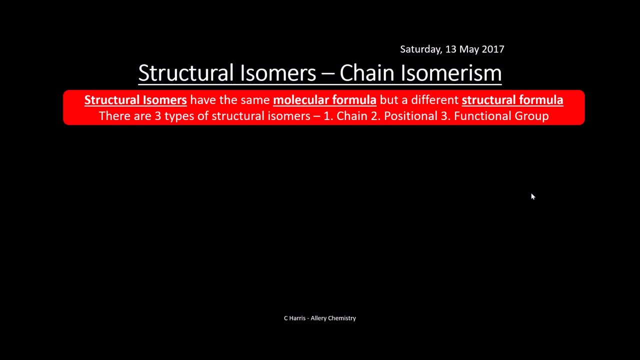 two um species, two radicals, which are the same, obviously, one's x dot, one's y dot. okay, structural isomers, uh, let's have a look at chain isomerism. okay, so structural isomers. basically, these have the um molecular formula, the same molecular formula as each other, but they're different. 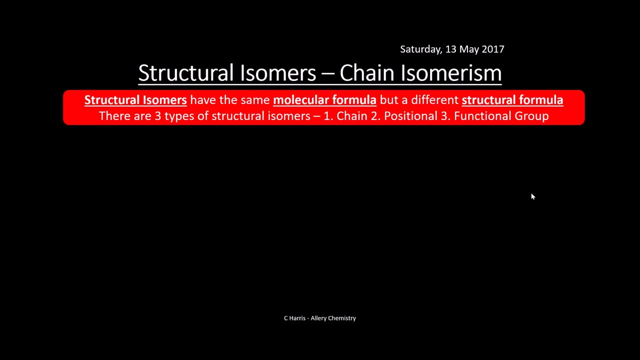 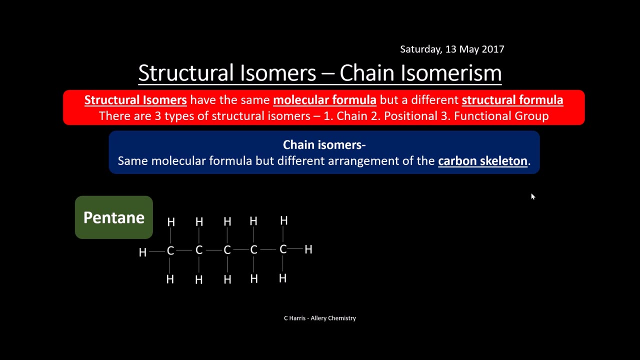 structural formulas and we need to know the three main types. we've got chain, positional and functional, so we're going to look at chain first. so chain isomers have the same molecular formula but different arrangement of the carbon skeleton. okay, so let's have a look. pentane: here's an example. 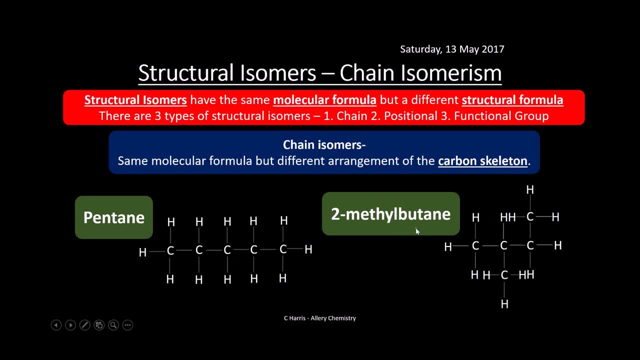 and two methyl butane. these are two isomers of each other. if you count the number of carbons and hydrogens, they will be the same in each molecule. however, this one has got a different carbon arrangement in its skeleton- carbon skeleton arrangement. you can see here we've got four here. 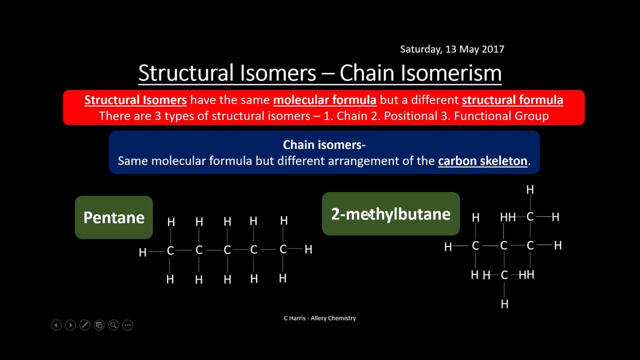 and a methyl group branching off the carbon skeleton. so we've got two isomers of each other. so this is two methyl butane, but the same molecular formula, different arrangement on the carbon skeleton. these are chain isomers of each other, positional isomers. these have the 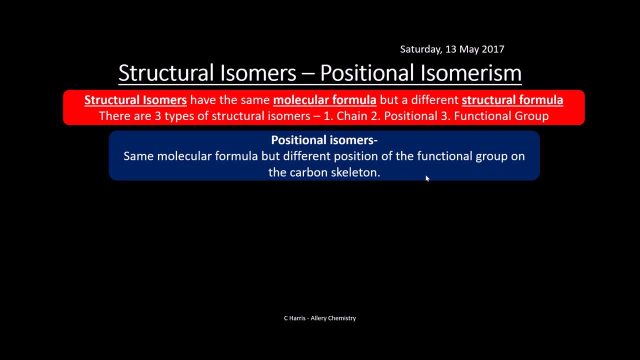 same molecular formula but a different position of the functional group on the carbon skeleton. so, um, this is obviously quite important, um, because you're going to see a lot of these within organic chemistry. so here's an example: pentane 1-ol. the alcohol group is obviously. 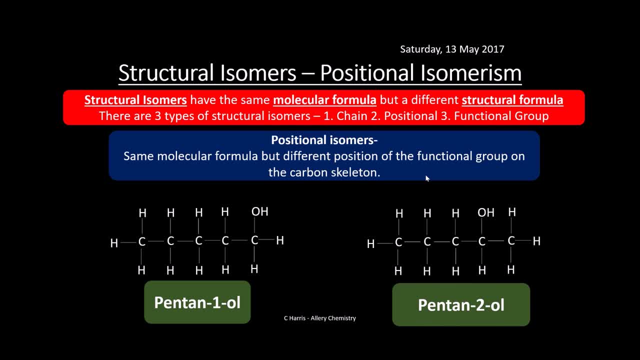 sitting on the first carbon skeleton and the second carbon skeleton is sitting on the second carbon and an isomer of that could be pentane 2-ol. so pentane 2-ol is an alcohol group now sitting on the second carbon. so this has changed its position. it's a positional isomer. 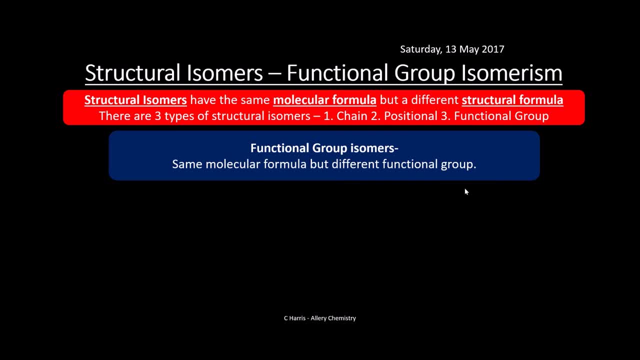 okay. functional group isomers: these have the same molecular formula but a different functional group. okay, so these are a little bit trickier. so let's have a look at an example. this is pent 1-ene, and you can see that we've got five carbons here, okay, and 10 hydrogens. this is pent 1-ene and this is.